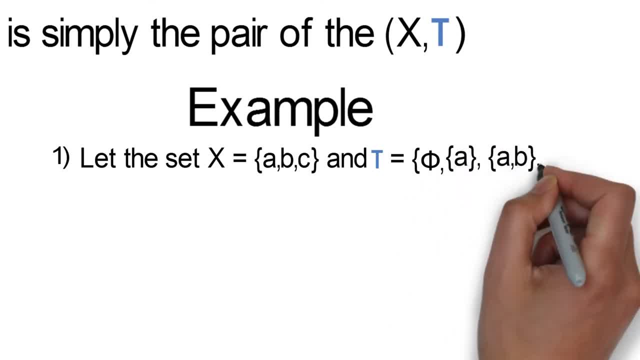 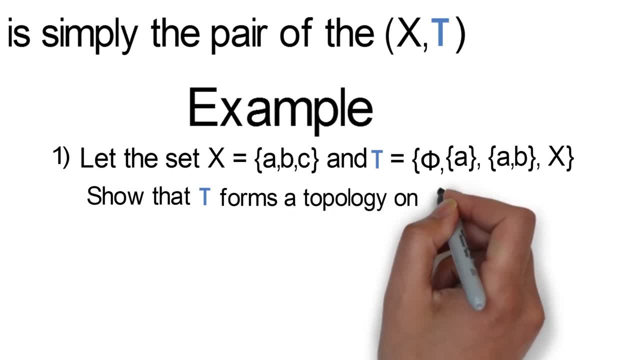 A, the set A and B and the set X Now show that tau forms a topology. on X Solution. Now we show that tau satisfies the three conditions of a topology. Condition 1 states that tau contains elements A, B, C and tau contains the set of an enterset. 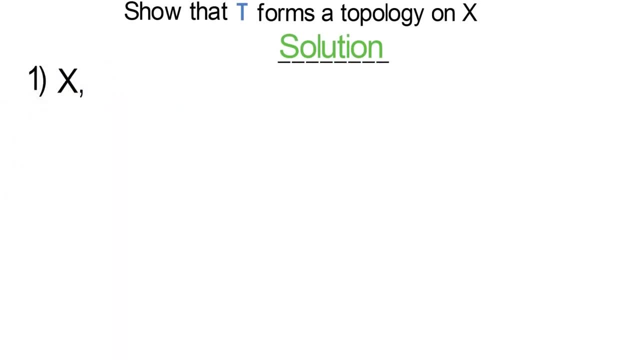 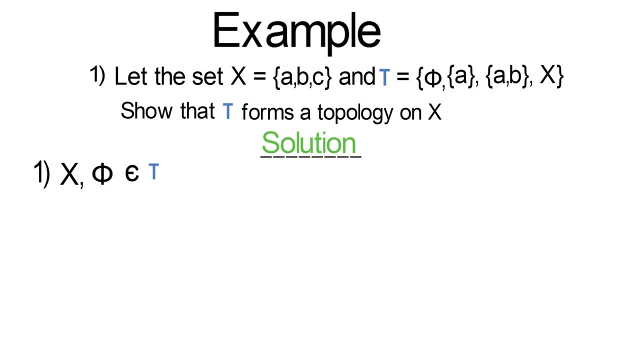 the simulating set A, the set A and B and the set X. We can see that the entire set X and the entersets are elements of tau. We can see that this is true from the given elements of tau in the question. So condition 1 holds. 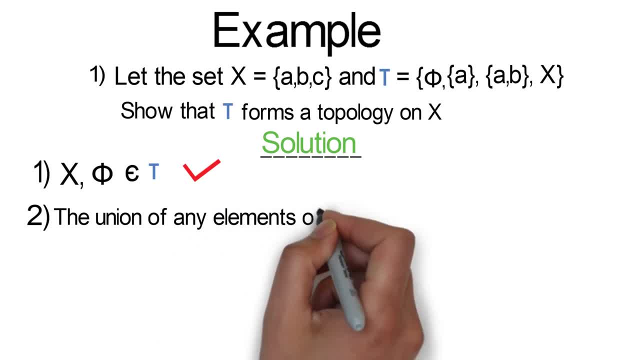 Condition 2 states that the union of any elements of tau is also a member of tau. Let's take any two elements from the set tau and find their union. So the union of any elements of tau is also a member of tau. The union of the simulating set A and the set A B. 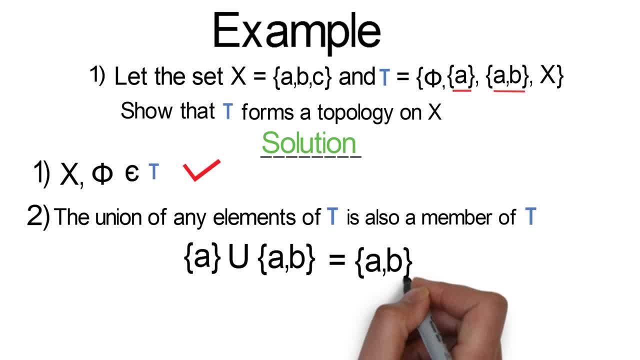 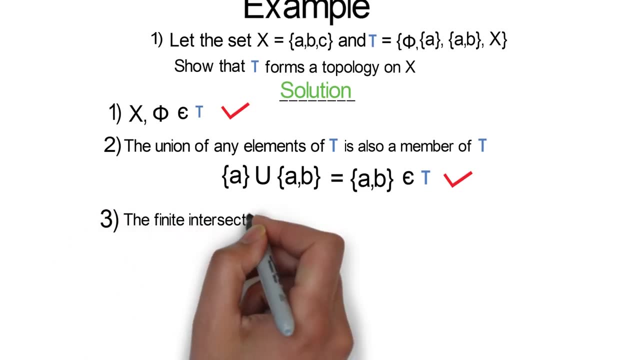 We have the set A B when we find their union, And the set A B is also a member of tau, So condition 2 holds. What about condition 3?? It states that the finite intersection of any member of tau is also a member of tau. 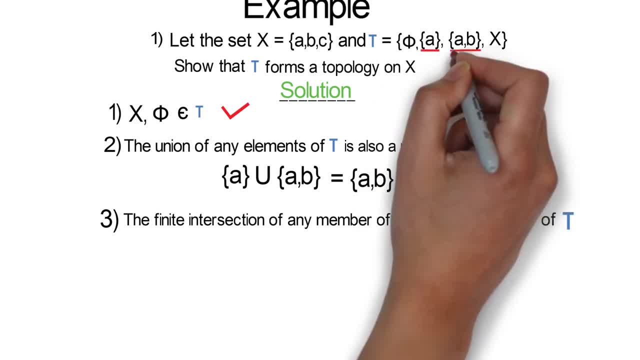 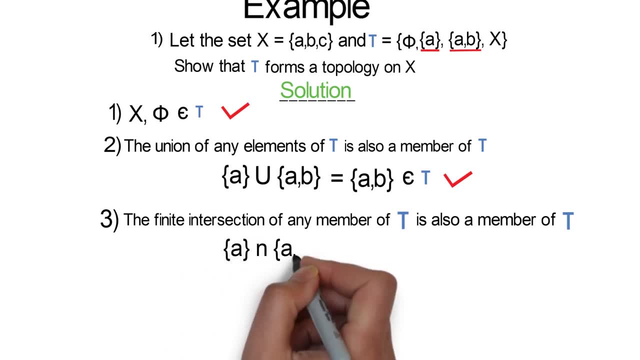 Let's take two elements of tau and find their intersection, Finding the intersection of the simulating set A and the set A B. we have a simulating set A Which is also a member of tau, So condition 3 also holds. 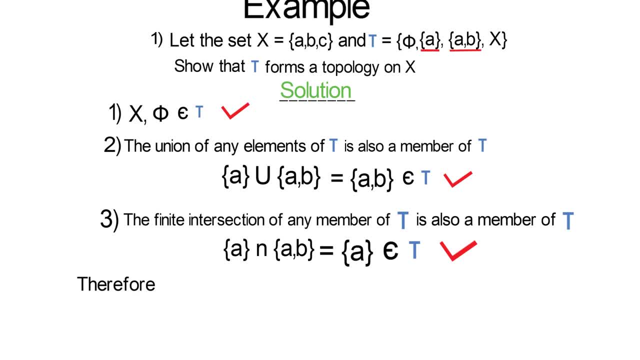 Therefore, we can finally say that tau is a member of tau. So we can say that tau is a topology of x. I also like to say that you are free to try out every other element in tau. Try to find their intersection, Try to find their union. 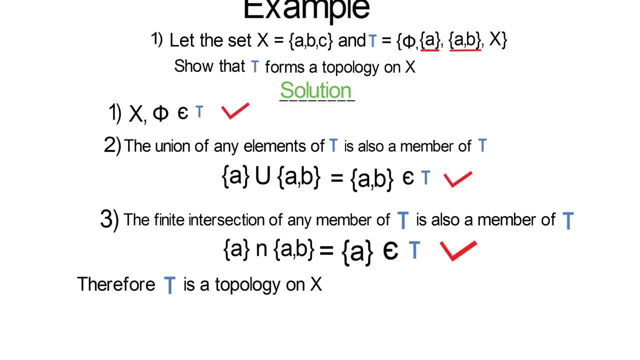 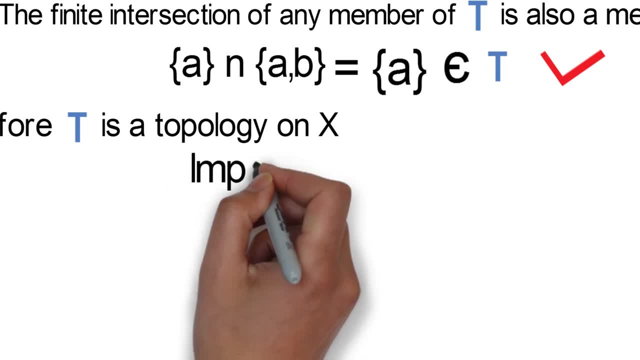 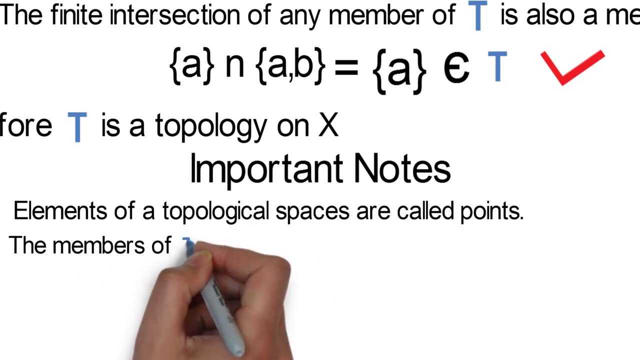 You will all see that they will all be an element of tau, Which proves that this is a topology of x. So take in some important notes: Elements of a topological space are called points And the members of tau are called the insets of a topological space.